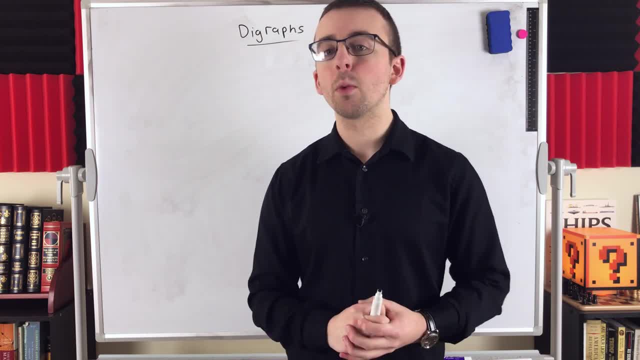 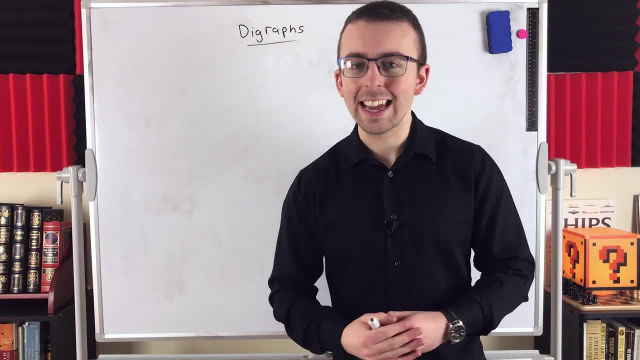 like a reasonable development right. There are some situations we might want to model with graphs, but in order to accurately represent them, we would need to use direction in the edges. So let's begin. We'll look at a undirected graph and we'll see how that compares to a directed graph. 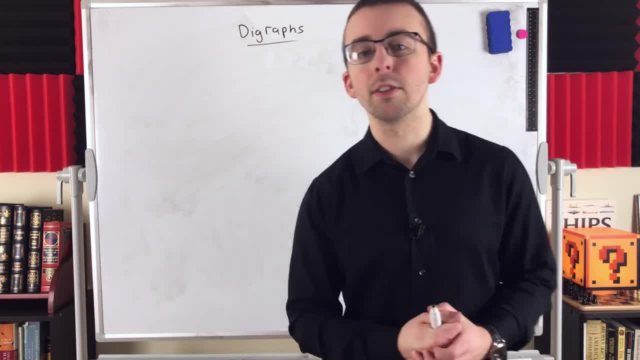 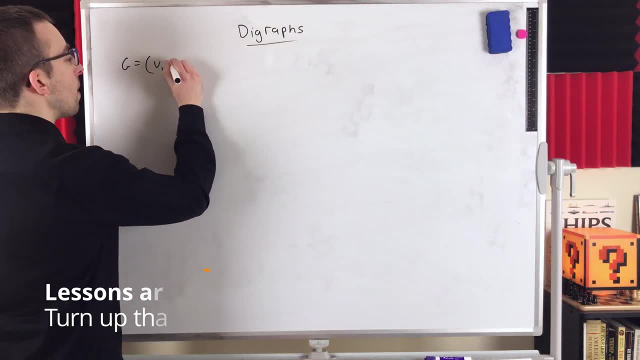 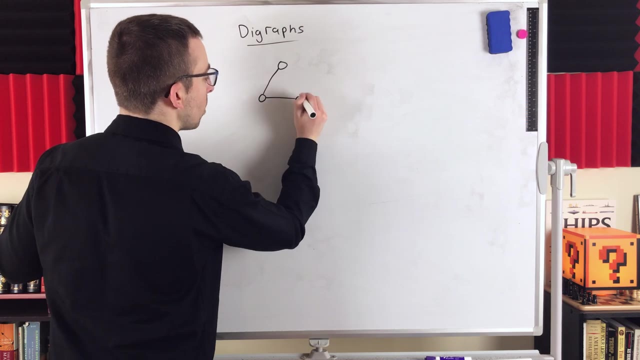 where some of the differences are and some of the language that we use to describe directed graphs. You're probably familiar with the fact that a graph is an ordered pair with a vertex set and an edge set. Here's an example of an undirected graph, which we will shortly. 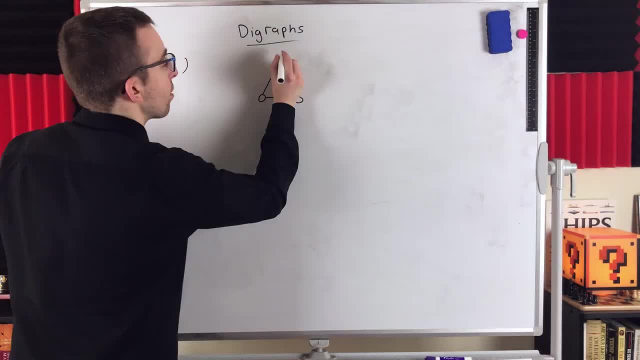 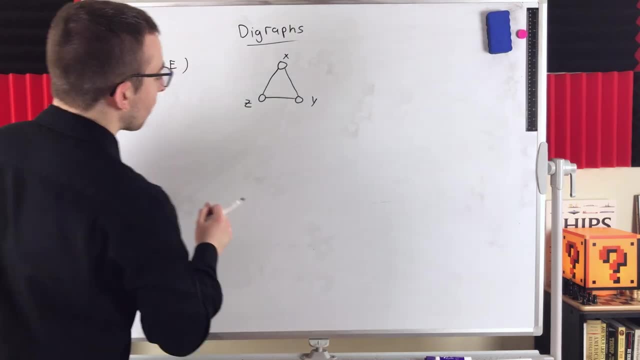 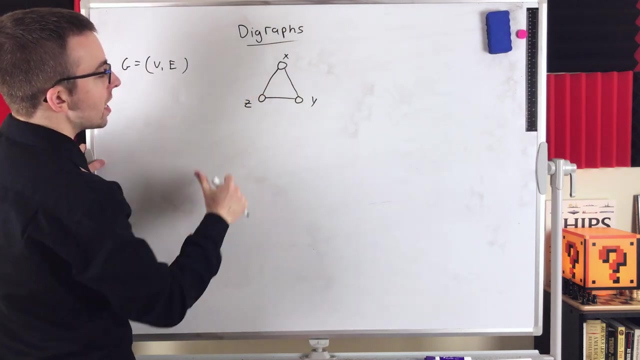 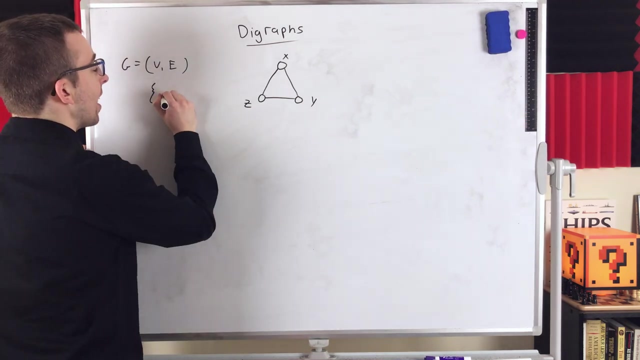 turn into a directed graph. Say it's got three vertices: x, y and z. In the case of an undirected graph we define an edge to be a two-element subset of the vertex set. For example, this edge here joins the vertices x and z. So we can describe that edge with this two-element set. 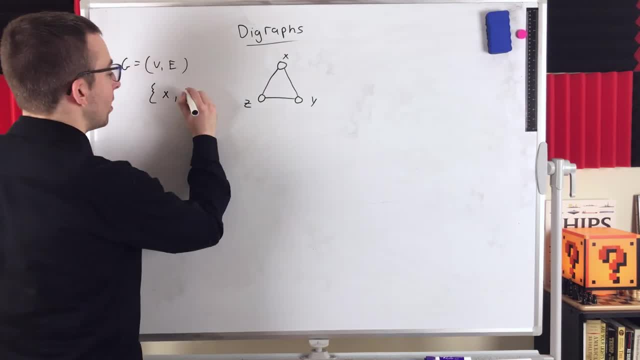 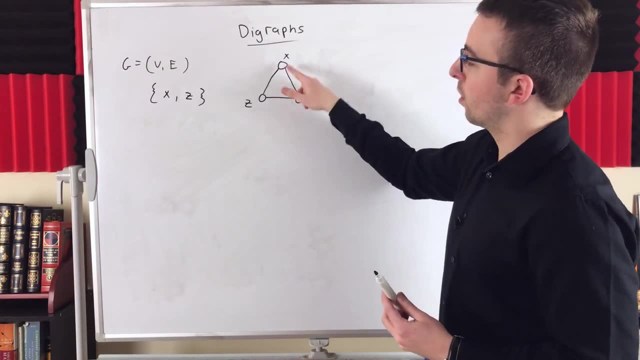 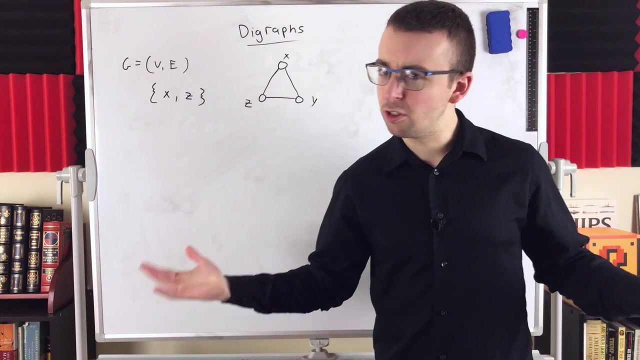 just a set that contains those two end vertices, x and z. That should seem reasonable, because there's no order in the description of this edge, right? It's just an edge that joins x and z. It joins z to x. it joins x to z. There's no order to be considered. 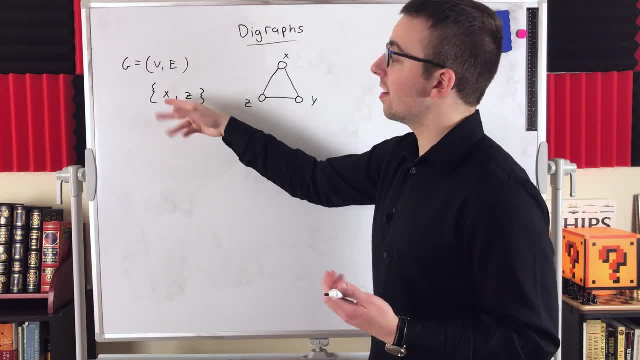 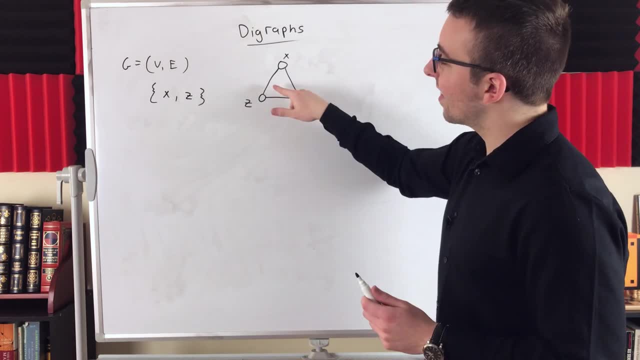 so it's perfectly fine to describe that edge with a set that contains its two end vertices. Things, of course, get a little bit different if we assign a direction to these edges. Describing an edge as a two-element subset of the vertex set, we can define an edge as a two-element subset of the. 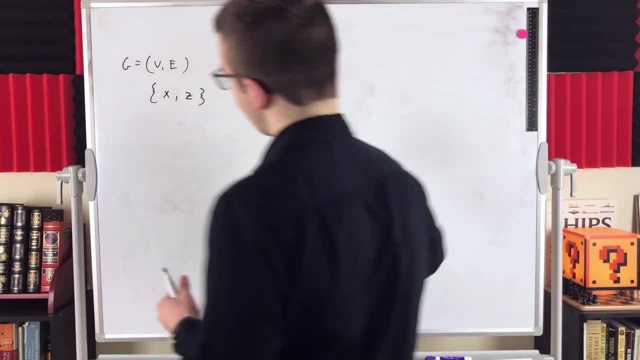 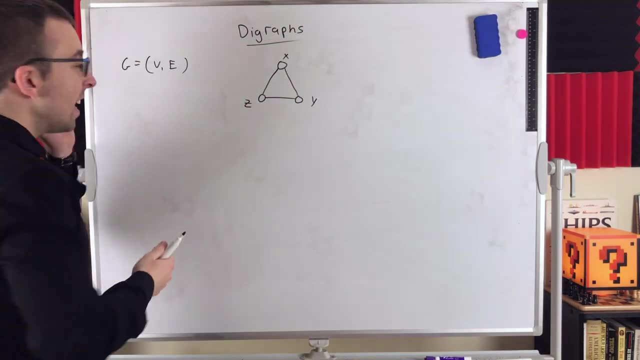 vertex set, but a pergi-text set won't cut it if we start to consider direction. So let's see that in action. Also, for an example of a situation where we might make this change, this graph could represent teams who have played each other in some sort of competition. 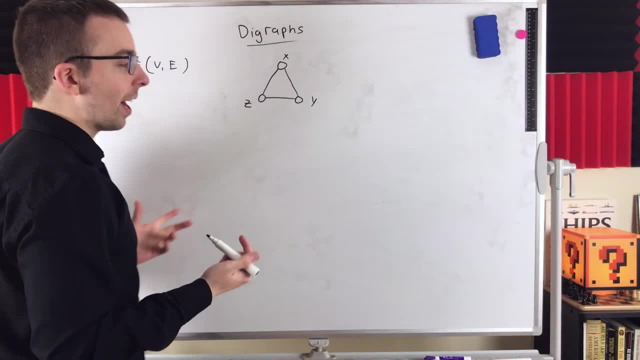 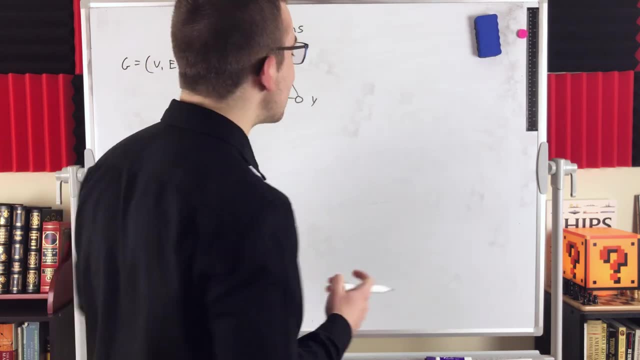 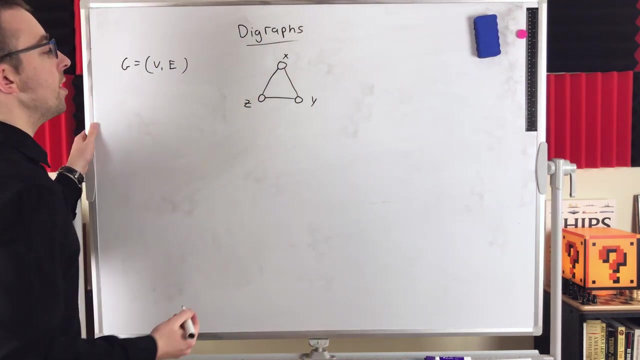 So Team X has played Team Z, Team X has played Team Y, and so on. But what if we want our graph to represent the team who won in that competition? Then we could use a directed graph, we could use directed edges. So check this out, Let's assign a direction to these edges. 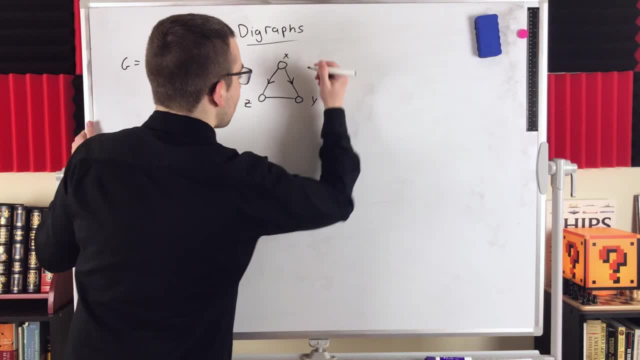 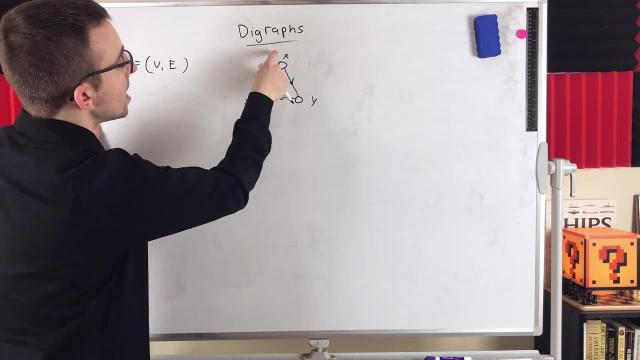 I'll do it with a nice arrow in the middle of the edges. So this tells us there's an edge from x to z. So we could say team x beat team z. There's an edge from x to y: Team x beat team y. And. 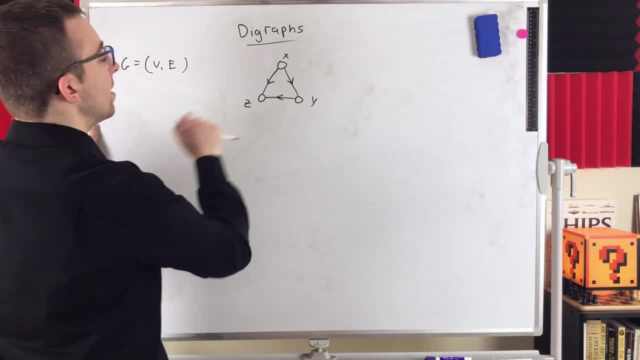 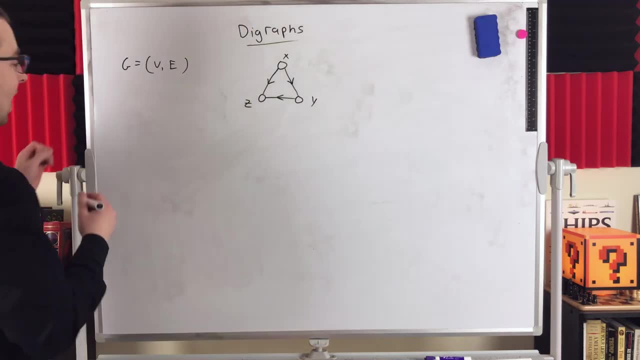 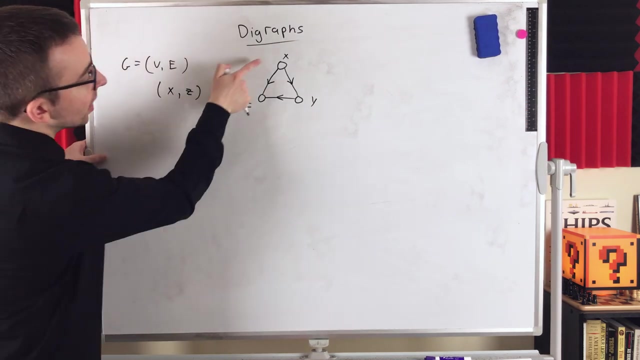 there's an edge from y to z, So team y beat team z. Now how do you think we're going to define an edge in a directed graph? One of your first guesses might be an ordered pair, And that's exactly right. So the directed edge going from x to z can be described with this ordered pair. 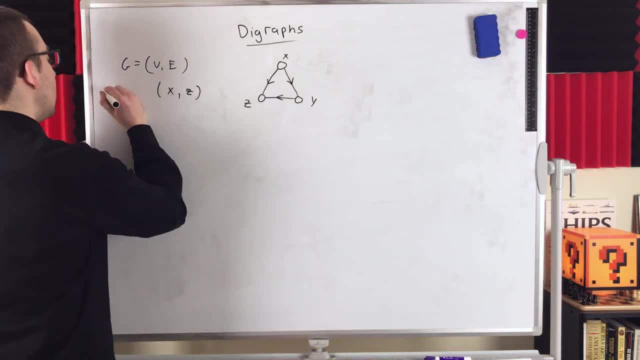 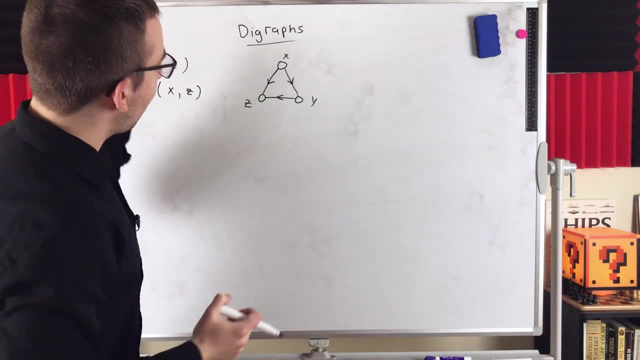 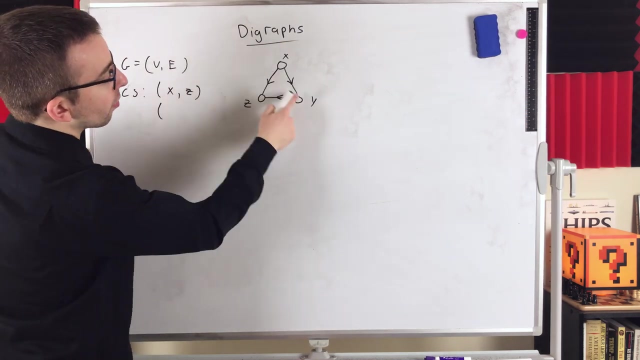 that has x first and z second. We call these directed edges- or another name we use, which I kind of prefer- Arcs. We call them arcs of a directed graph. So what are the other two arcs of this graph? Well, we've got one more arc going from x to y And then a third arc going from y to z. 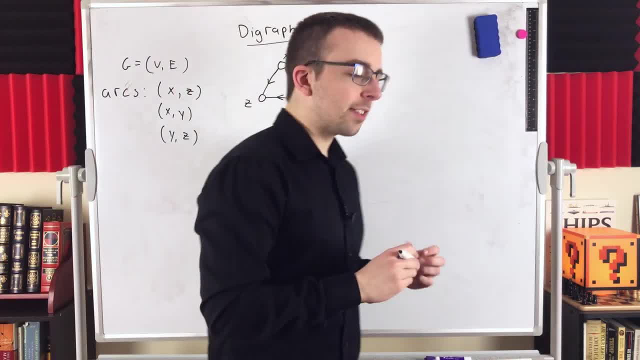 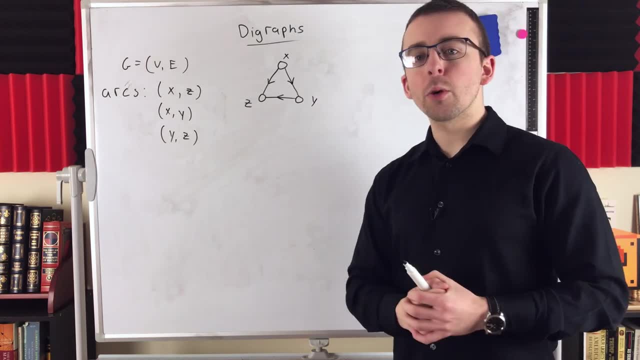 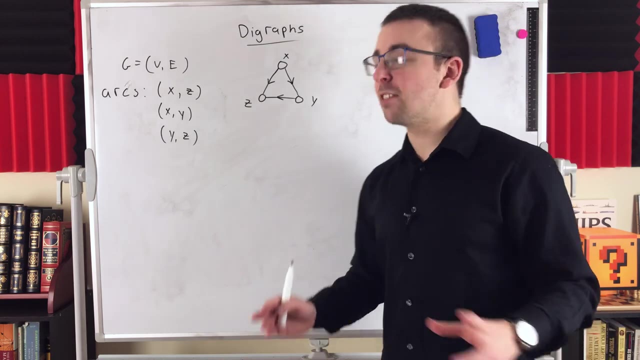 Pretty cool. So there are a couple things to consider here with how this relates to an undirected graph. A lot of the definitions you might be familiar with about things like trails, walks, paths, Cycles, Circuits- All that stuff is really similar. It's defined in a really similar way. 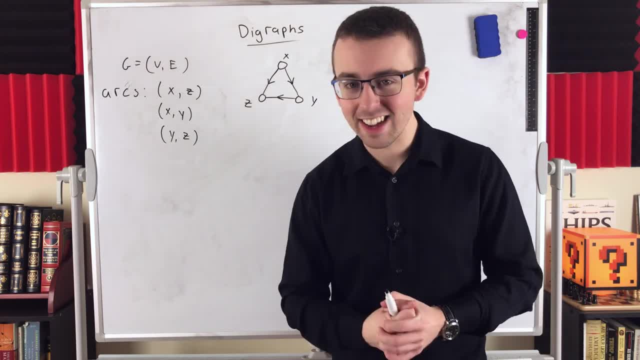 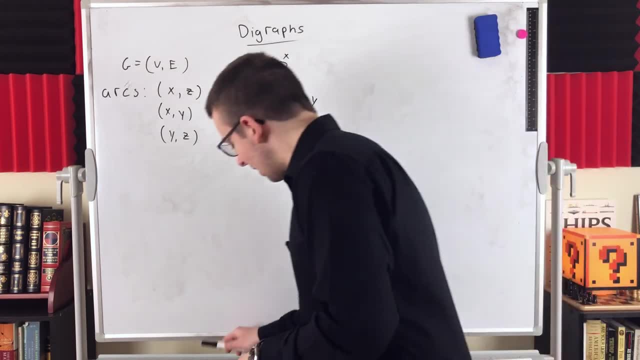 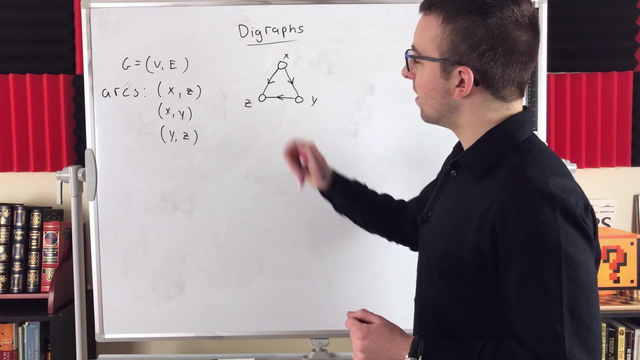 for a digraph, Pretty much exactly how you would think they would be defined. Let's see an example of a walk in this digraph. I'll go ahead and change my color. Maybe I'll pull out the pink. I think the pink shows up well enough, So let's try the pink. Can you see a walk in this digraph from x. 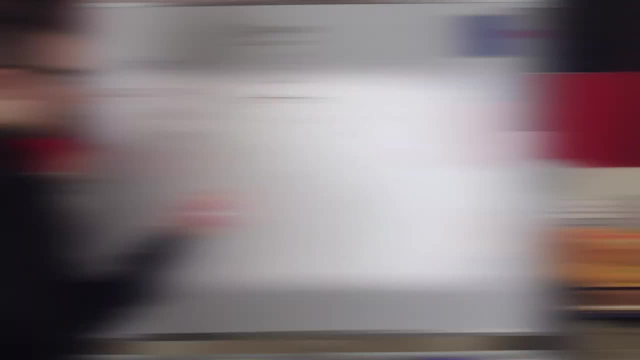 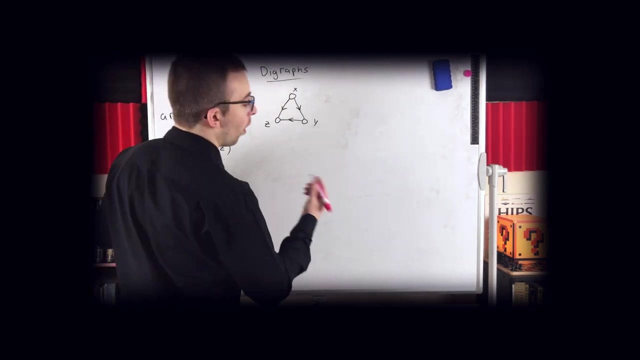 to z. Of course, There's two of them, in fact. What I said in the original recording at this time was wrong, so you're hearing this instead. Now that I'm done saying things that are wrong, let's take a look at a walk. 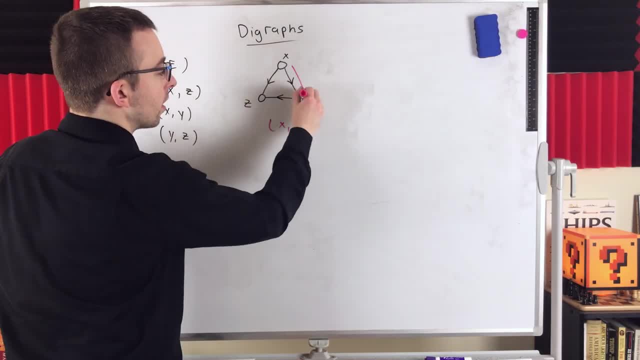 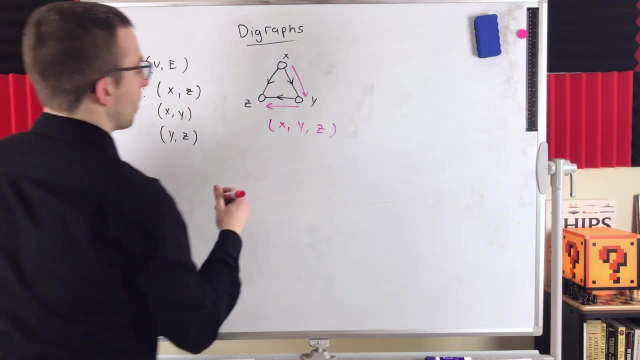 We could start at the vertex x, Then we could go to the vertex y, And then we could go to the similar one. That is our destination. So that's a walk from x to z, And as we, Wasserán takes us up. 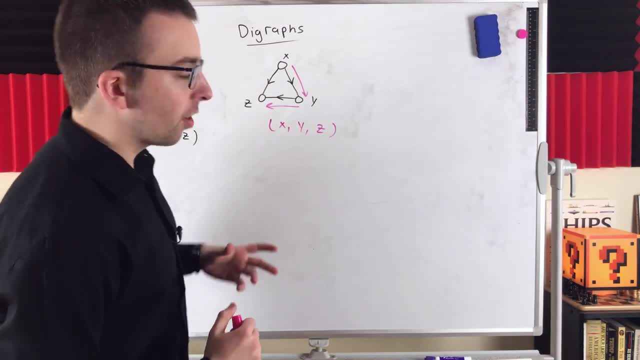 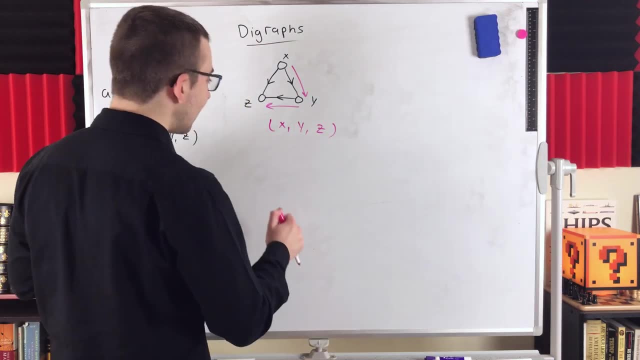 So that's a walk from x to z? No, it turns out that is also a path, path from x to z, by definition of a path, because we're not repeating any vertices or edges. On the other hand, now in an undirected graph, since there's a path from x to z, there's 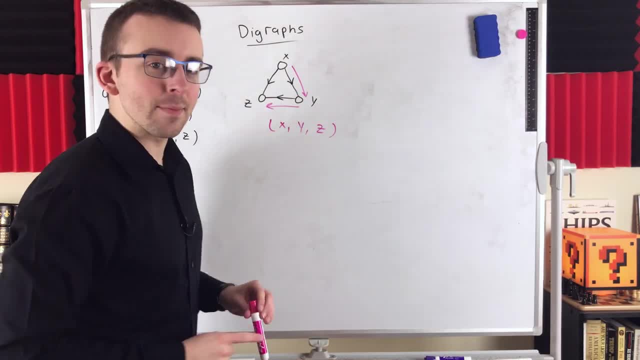 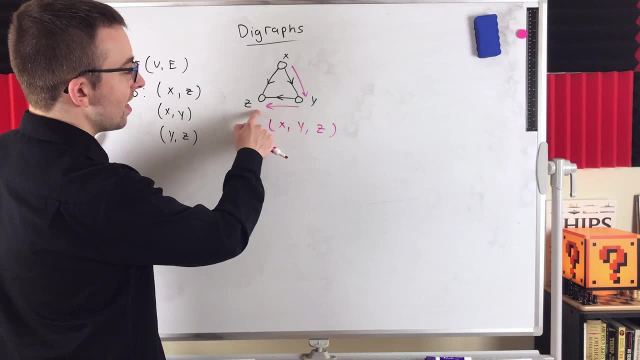 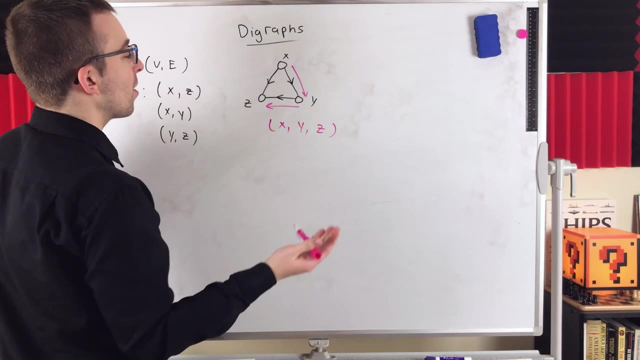 certainly a path from z to x. right, You could just go the other way, But in a directed graph that's not always going to be the case. Is there a path or a walk from z to x in this directed graph? No, As you can see, if we start at z, we can't go anywhere. There's. 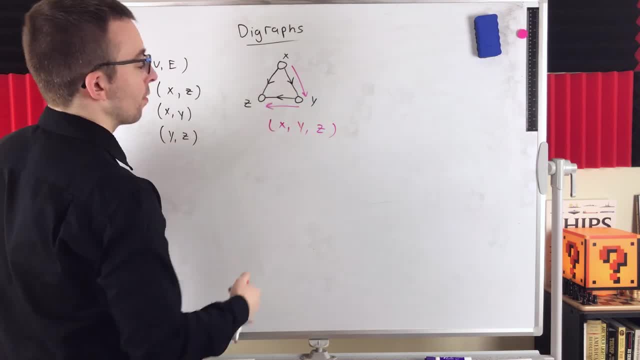 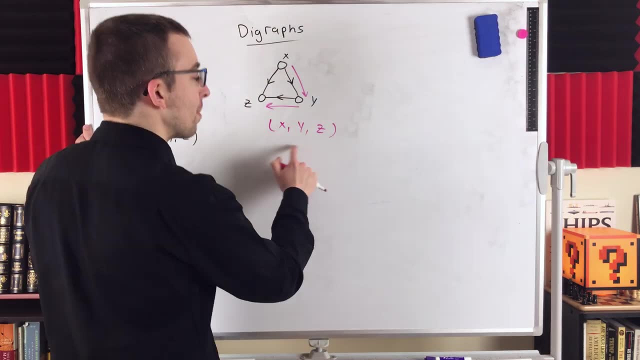 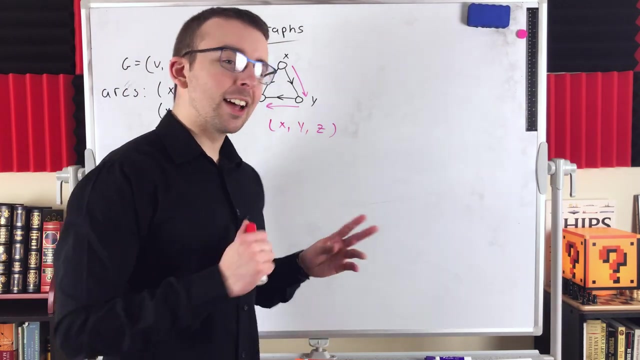 no edge, leaving z and going to any other vertex. So if we start at z, we're stuck at z, We can't get anywhere else. So there is a path from x to z, There's not a path from z to x. So that's kind of weird. So I think that observation definitely tells us that there. 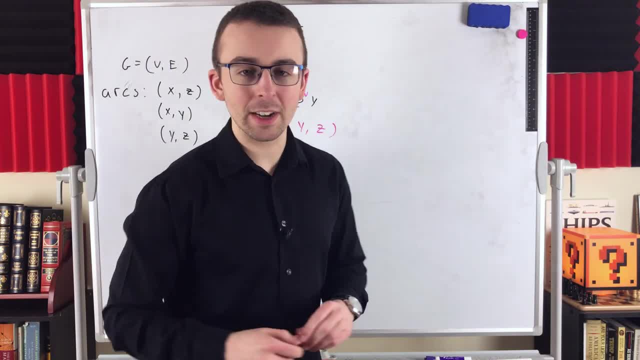 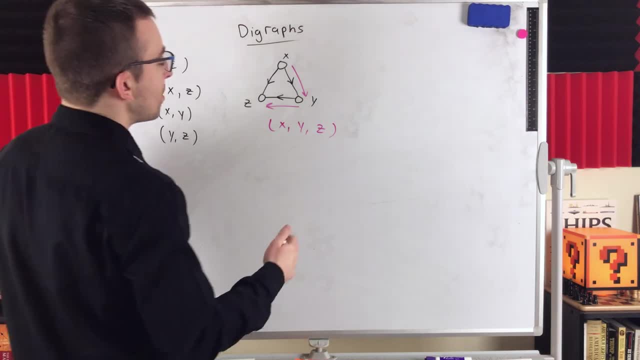 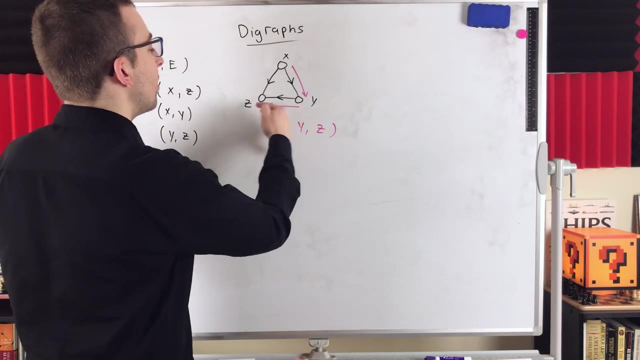 is a lot to be learned about digraphs. They definitely have their differences. It also touches on the idea of degrees of vertices in digraphs. Remember we said that if we start at z, we can't get anywhere. There's no edges leaving z, But there are edges going to z. 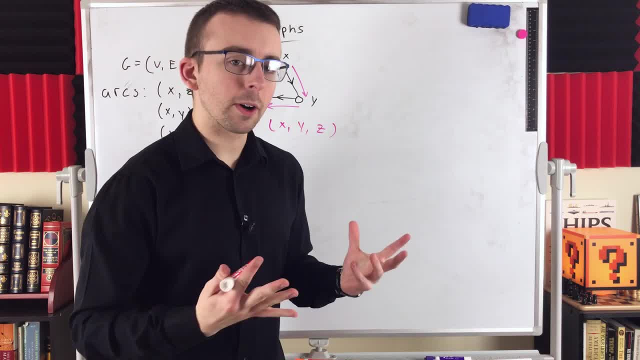 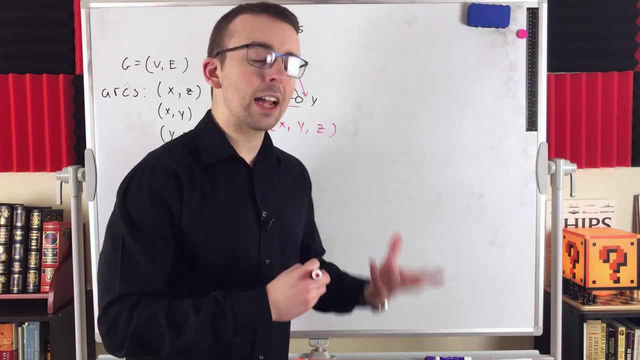 So that makes us think about degree. How do we define the degree of a vertex in a directed graph? Well, before we talk about that, let me just introduce some of the language we use to describe adjacent vertices in a digraph. Okay, 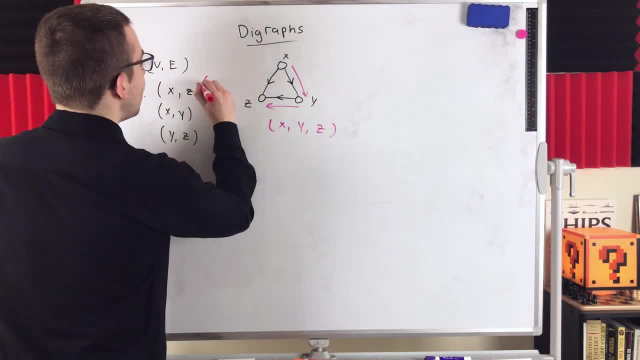 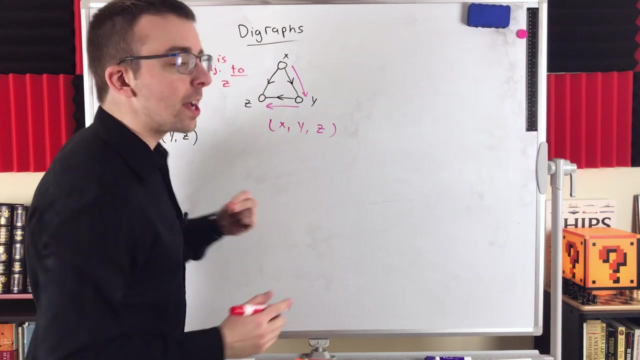 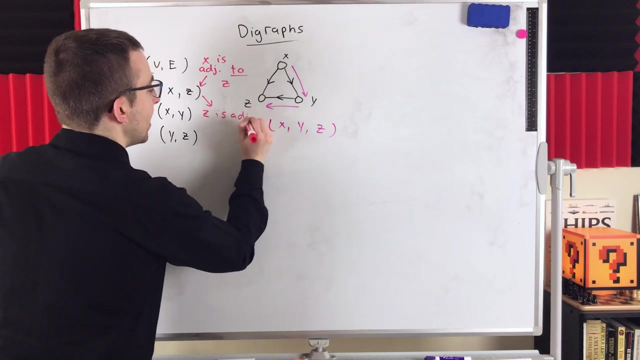 So, for example, if we have a graph, because there's an arc going from x to z, we say that x is adjacent to the vertex z, whereas z is adjacent from the vertex x. So I'll write that here: Z, the vertex Z, is adjacent- again abbreviated Adj: Z is adjacent. 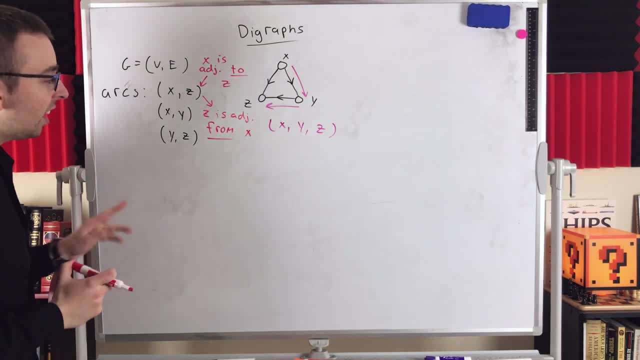 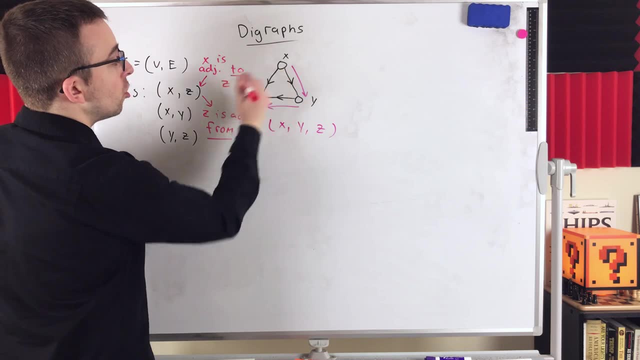 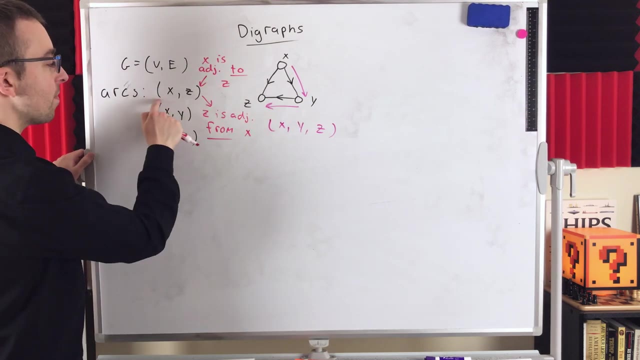 from the vertex x. If we said that z is adjacent to x, that would mean there's an edge going from z to x, but there is not. There's an edge going from x to z. So we say x is adjacent to z. 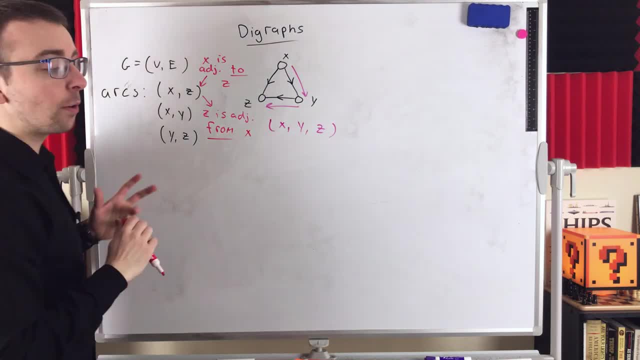 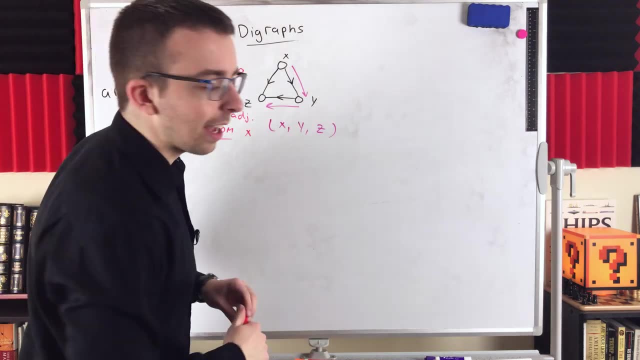 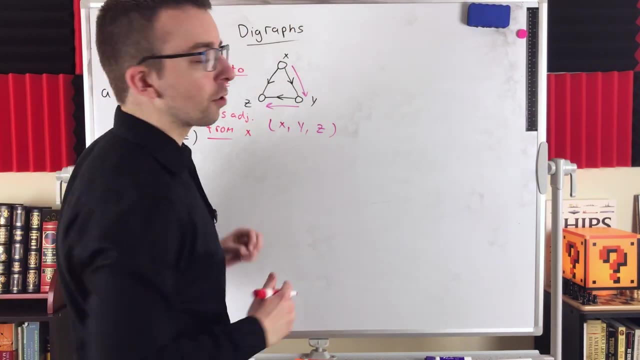 whereas z is adjacent from x. Now it's possible that z could also be adjacent to x, but in this graph we've drawn that's not the case. So now we can talk about the degree of a vertex in a directed graph. There's two types of degrees in a directed graph. First one we'll talk about is the. 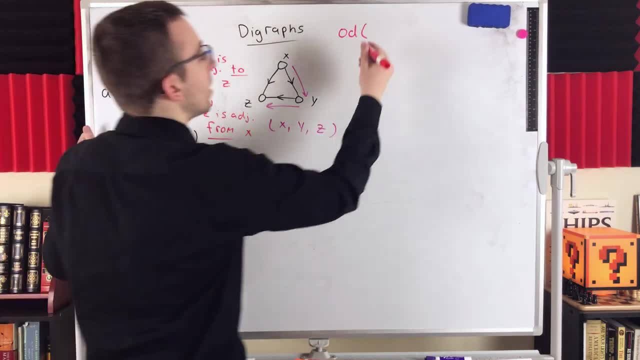 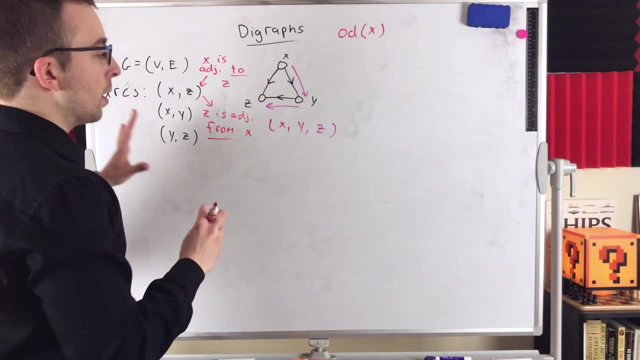 out degree which we can write like this: od of the vertex x, for example. that is the out degree of the vertex x, And if we were considering multiple graphs at the same time, we might want to write in the subscript of od. 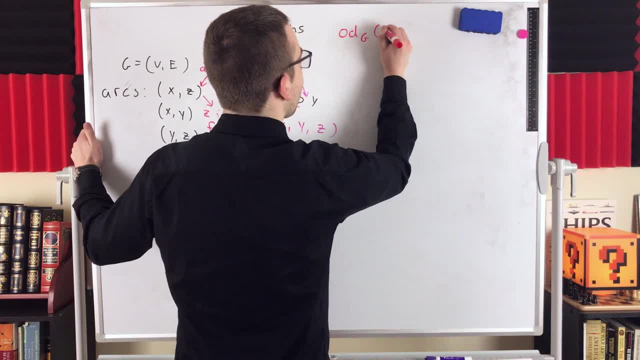 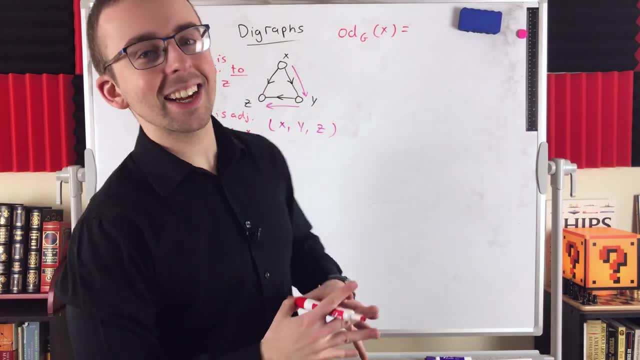 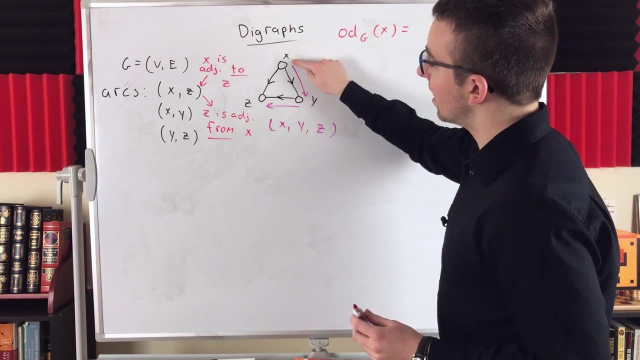 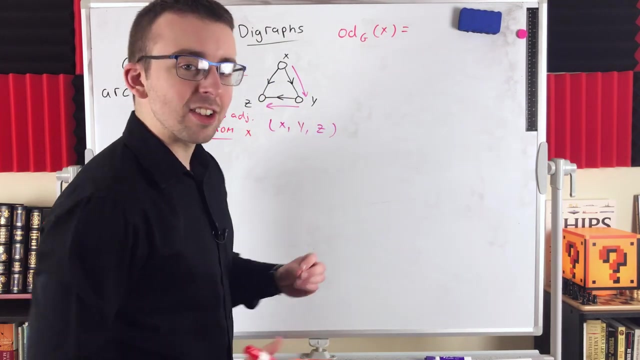 The graph we're talking about. So that would be the out degree of the vertex x in the graph g. The out degree of a vertex in a directed graph is the number of vertices. it is adjacent to x, is adjacent to two vertices. It's adjacent to z and it's adjacent to y. There are two edges. 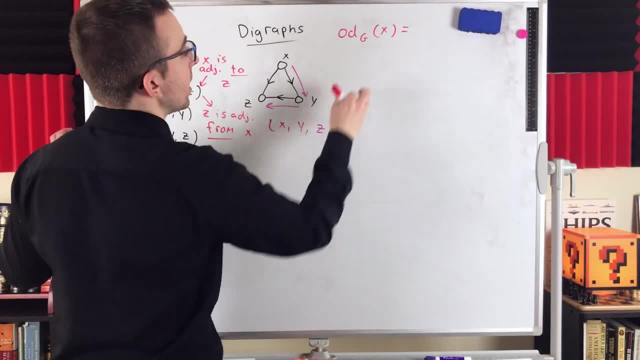 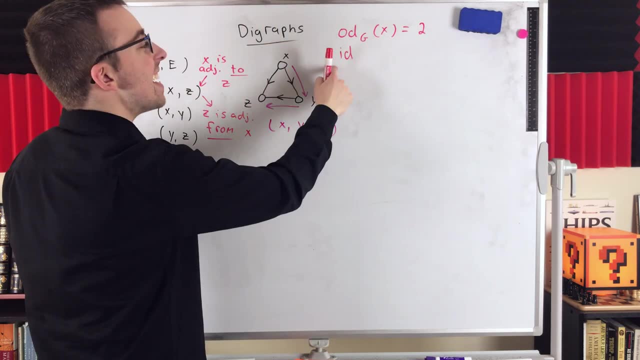 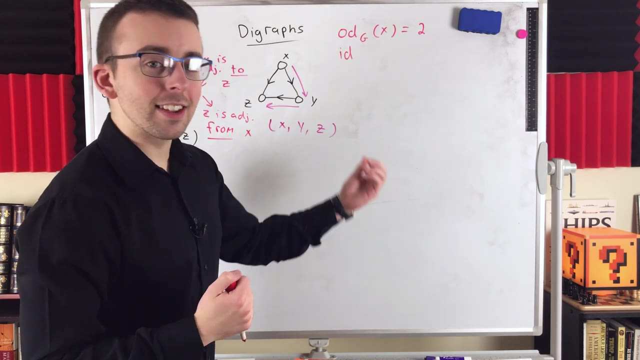 coming out of x. So the out degree of x in g is the out degree of the vertex x. The other type of degree, as you might have guessed, is the in degree. It's the number of edges coming in to a vertex or the number of vertices that a vertex is adjacent from. So for 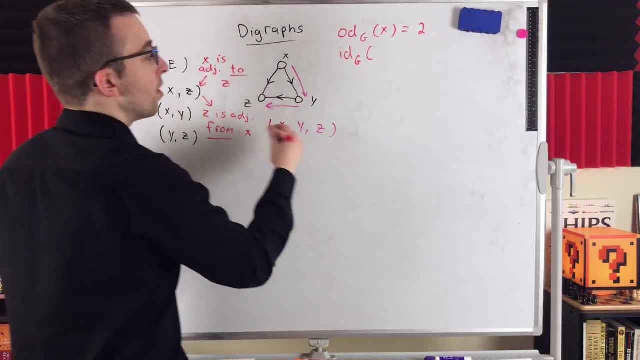 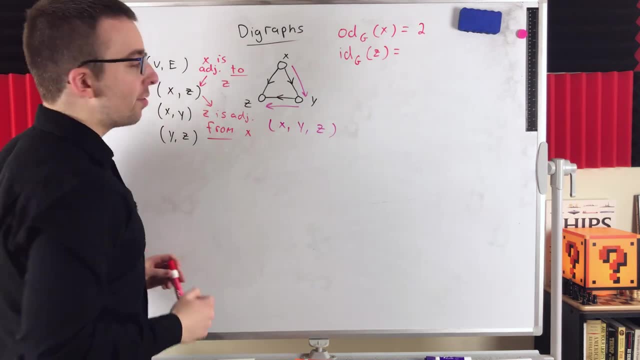 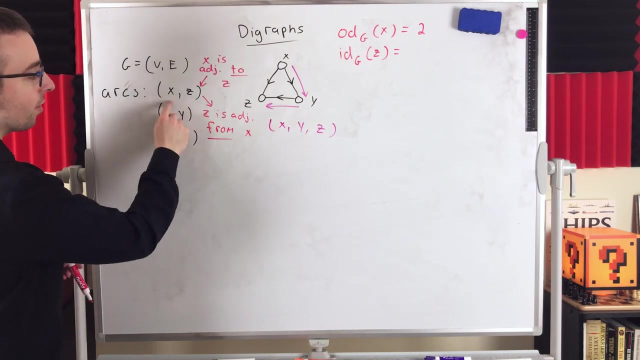 an example of in degree: the in degree of the vertex z in the graph g is equal to what? Well, z is adjacent from two vertices: The z is adjacent from y and z is adjacent from x, Or equivalently. again we can think about the edges. 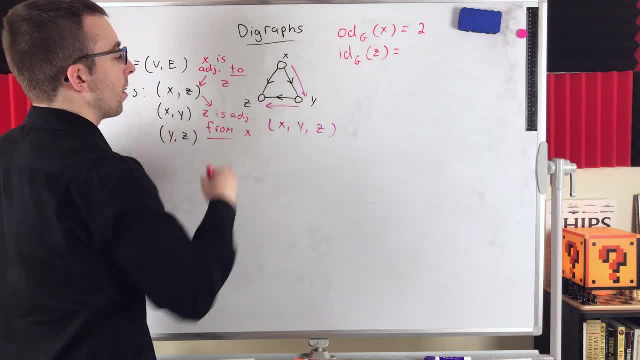 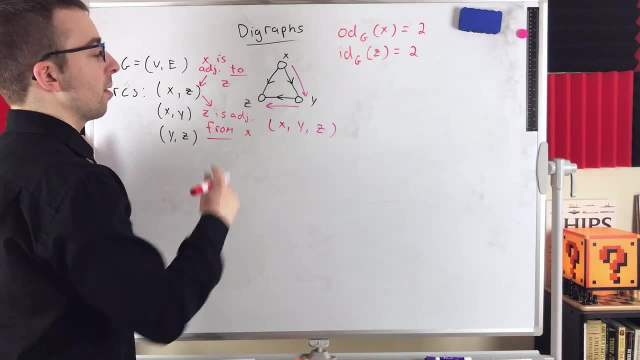 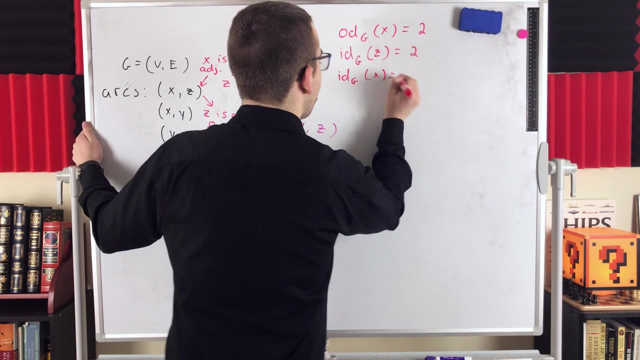 There are two edges going in to the vertex z, So the in degree of z is two. And if we describe the degree of these some of the other degrees as well, just for practice, what is the in degree of the vertex x? Well, we see there are no edges going into the. 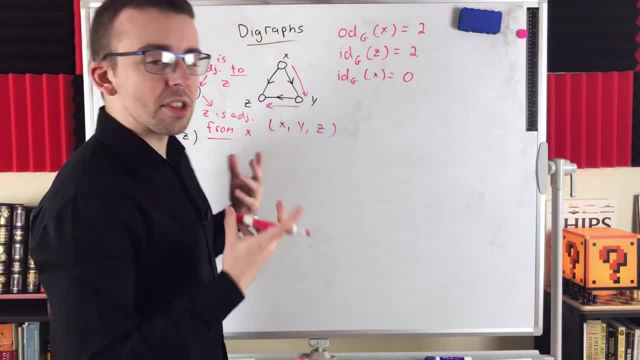 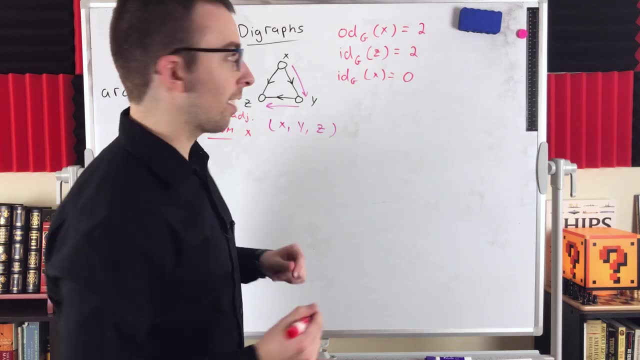 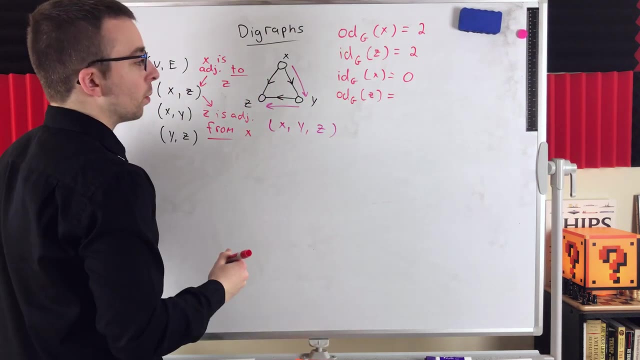 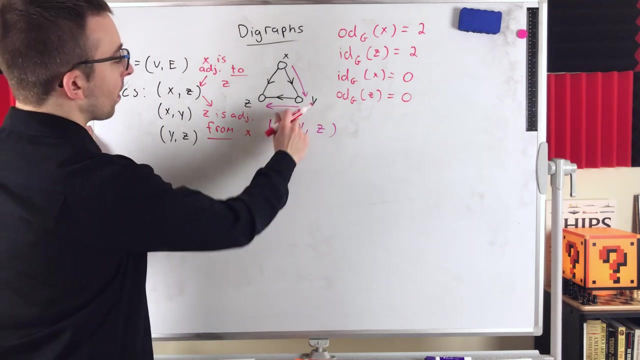 so the in-degree of the x is 0. And if we're thinking about this as modeling teams playing each other, that would mean that no team has beat team x. Similarly, the out-degree of the vertex z is equal to 0 in this case. So z has beat no teams. there's no edge coming out of z And then y. 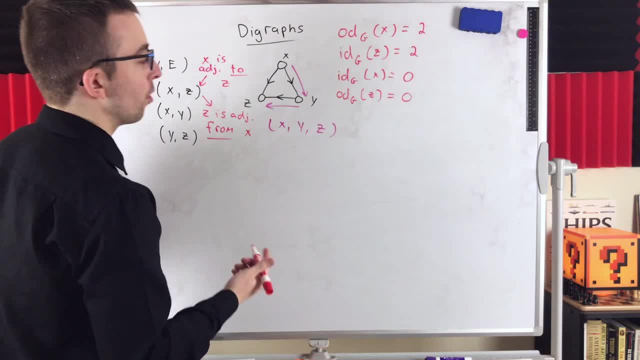 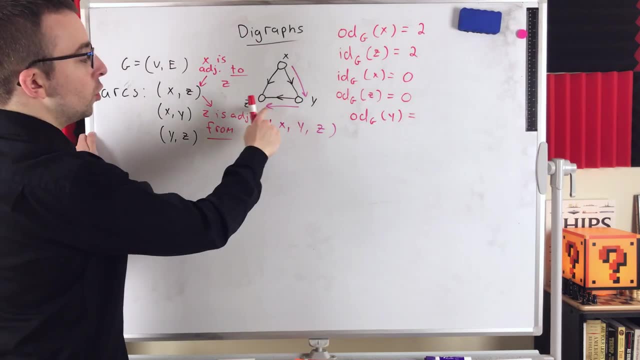 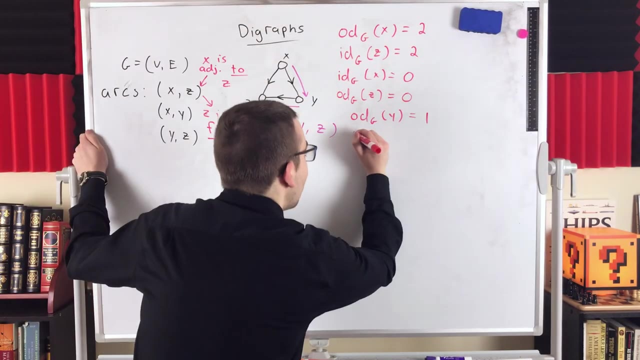 y is a little bit interesting because it doesn't have 0 for either of its degrees. The out-degree- the out-degree of y is equal to what It's equal to 1.. There's one edge coming out of y: y is adjacent to one vertex and the in-degree whoops. I just wrote i-n i-d. 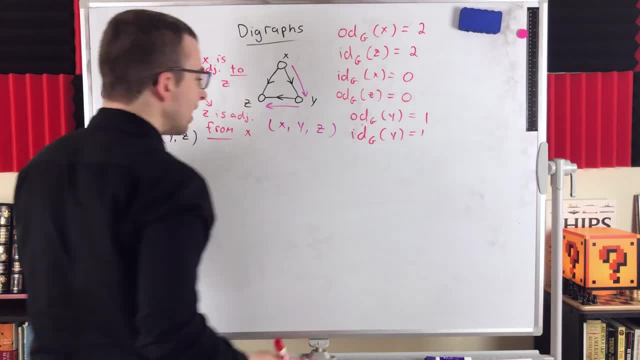 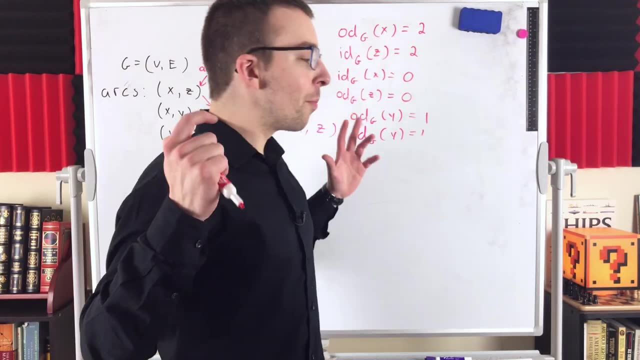 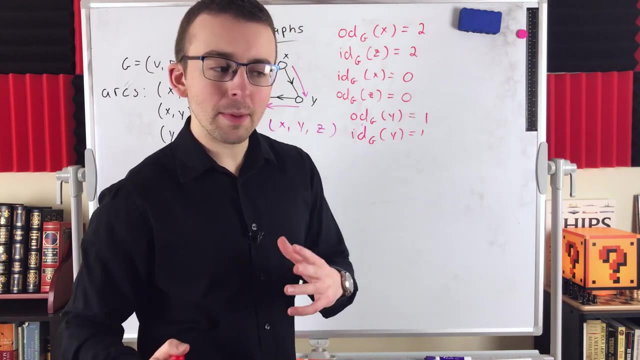 the in-degree of the vertex y is also equal to 1.. There's one edge going in to y, Oh man. So isn't that cool. I feel like we're opening up a whole new world. The directed graphs are really cool. I really like the sort of additional complications they bring about. that are really 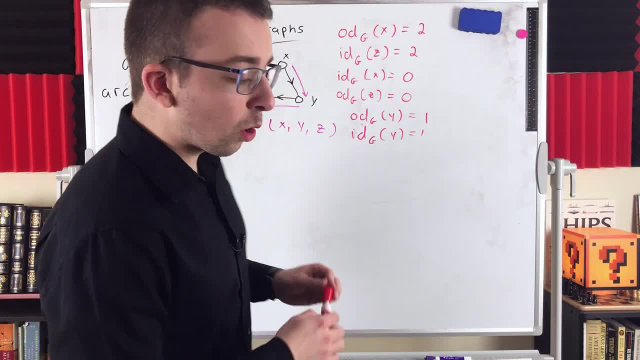 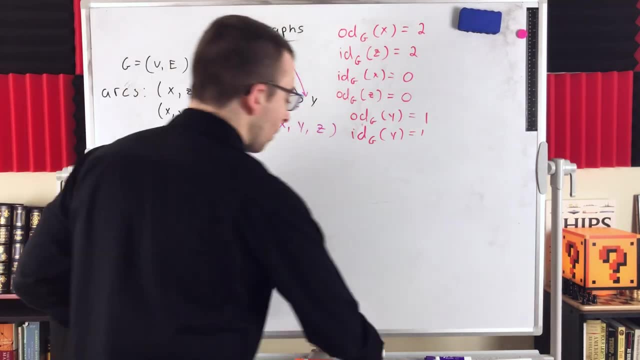 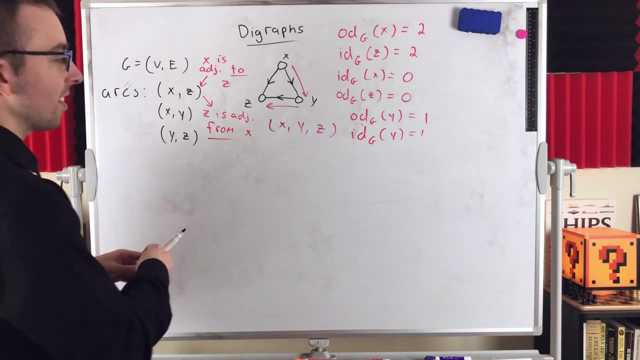 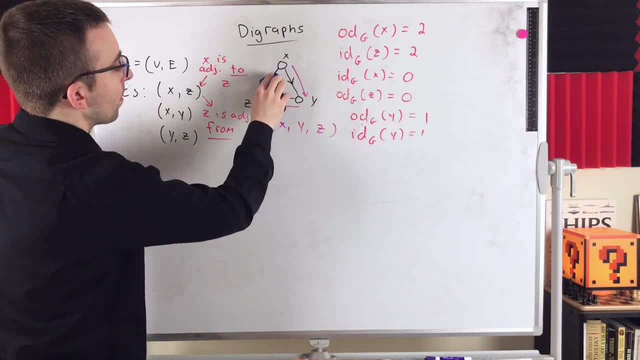 a diagraph And I'm going to draw a diagraph And I'm going to draw a diagraph And I'm going to, instead of x being adjacent to z, and that's it. let's imagine that x is adjacent to z. 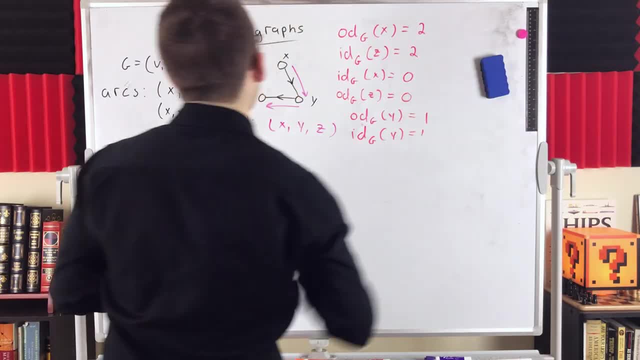 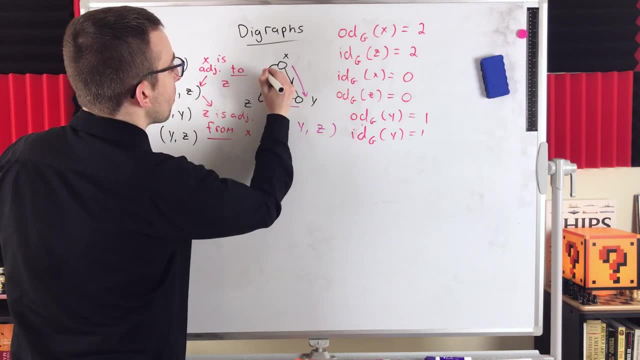 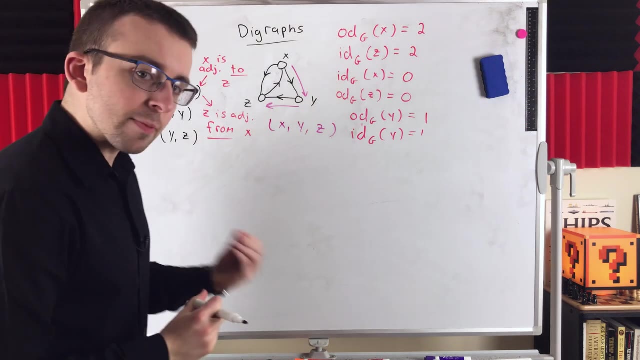 and z is adjacent to x. Now, one way we could draw that is like this: We could draw the edge or the arc, rather going from x to z and the arc that goes from z to x. So what I want to emphasize is that these are distinct arcs of a diagraph. They are considered 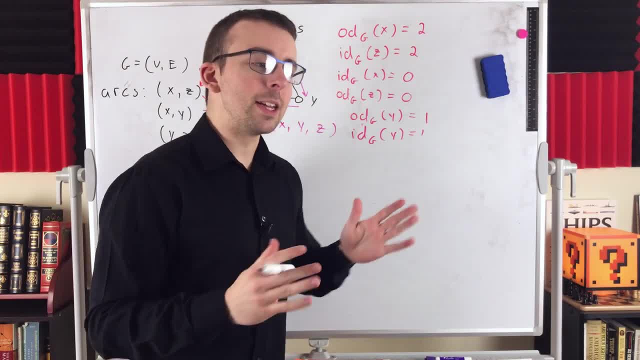 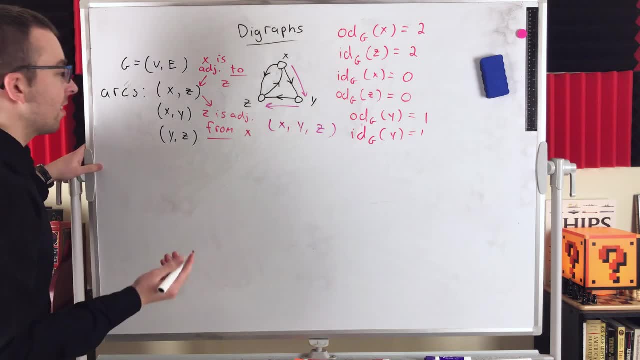 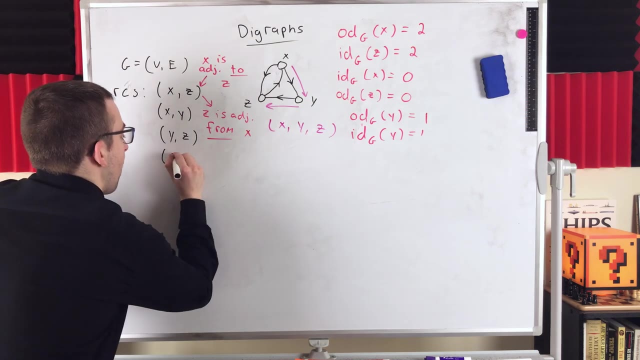 distinct arcs. They're not considered, for example, to be, you know, one arc that happens to go both ways. They're two distinct arcs, Which should make sense. you know, if we consider what an arc really is, One of these arcs is an ordered pair from x to z. The other arc is a different. 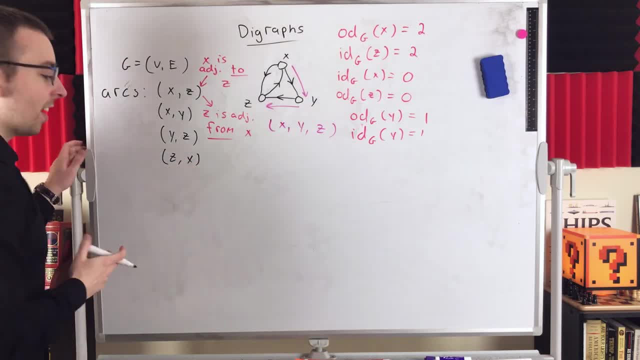 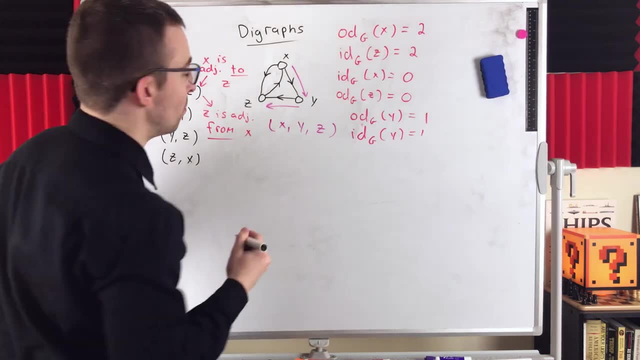 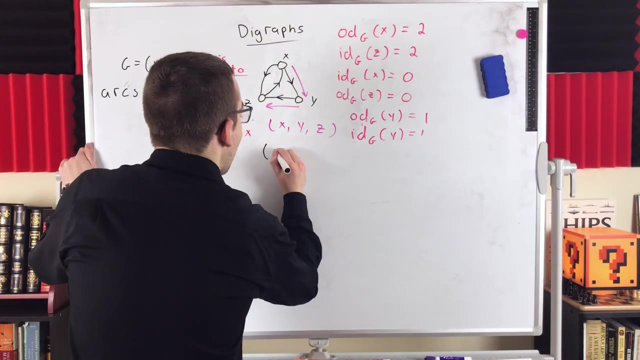 ordered pair. It goes from z to x. And then the last point that I think really emphasizes that is, we can make a cycle with those two arcs, which is very important. So let's say that we have a pretty sweet. We can make a type of cycle that never existed in undirected graphs, Going from x. 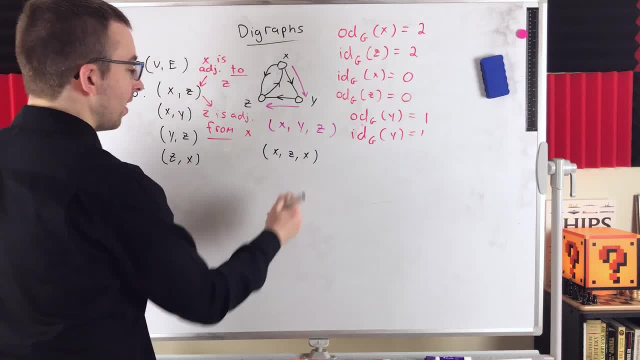 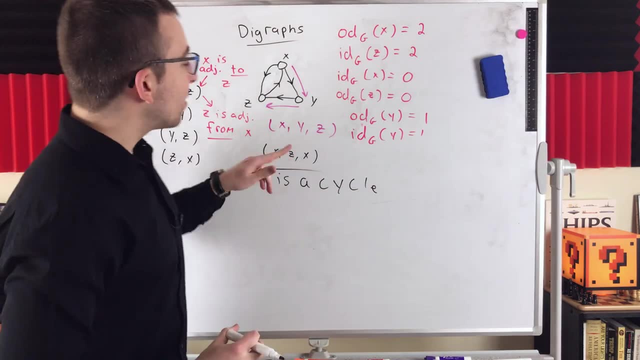 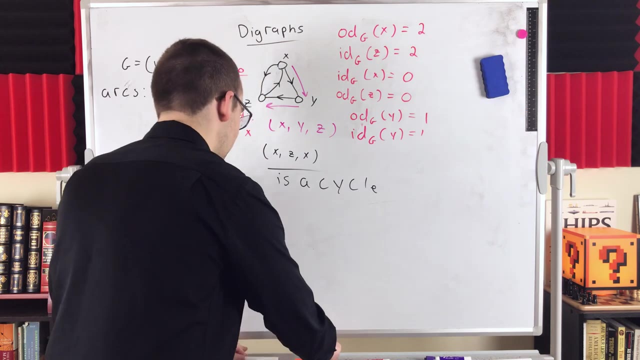 to z, back to x. this is a cycle. This is a cycle of this directed graph. It's only got two vertices, The cycle only has a length of two, but it is a cycle And let me use a different marker just to. 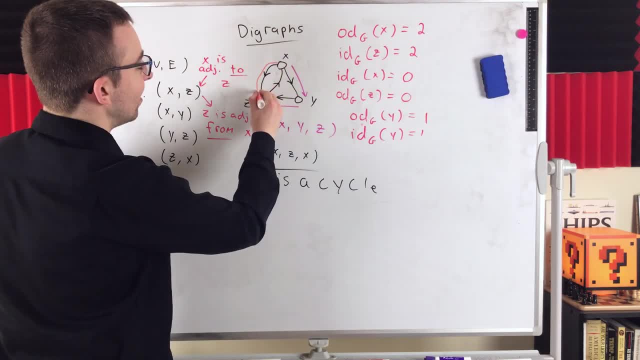 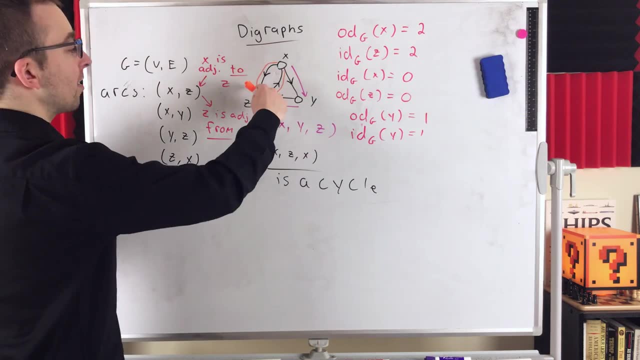 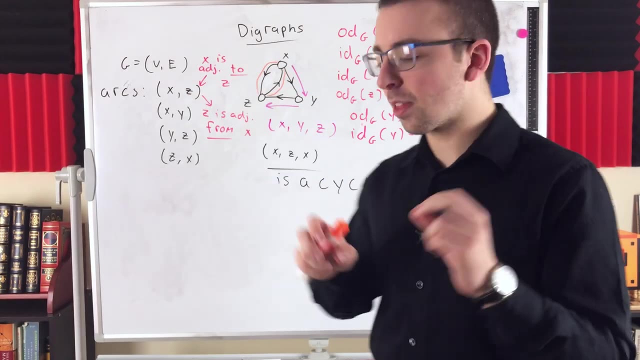 outline it. Look at that: Going from x to z, right back to x. pretty sweet, A cycle of length two. So the arc from x to z really is distinct from the arc that goes from z to x. Just want to emphasize that. Now, a couple things I want you to think about. 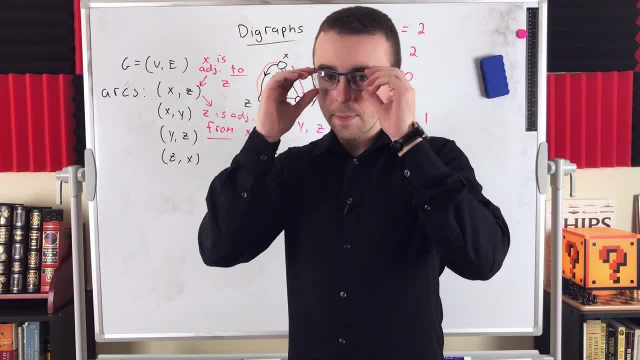 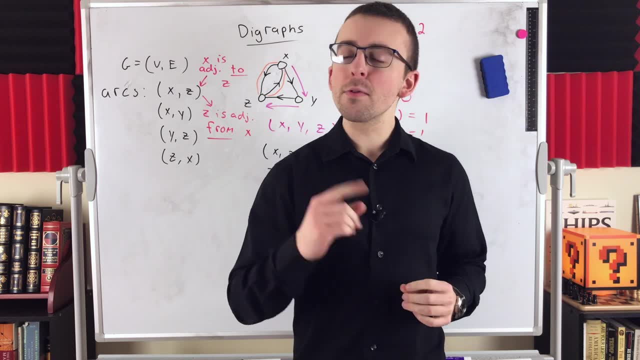 before the next couple lessons, Think about the idea of connectedness in digraphs. What does it mean for a digraph to be connected? One other thing you might remember: the first theorem of graph theory. It tells us that if we add up the degrees of the graph, we get the degree of the. 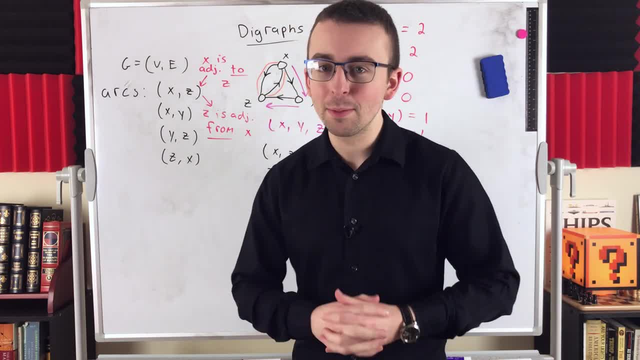 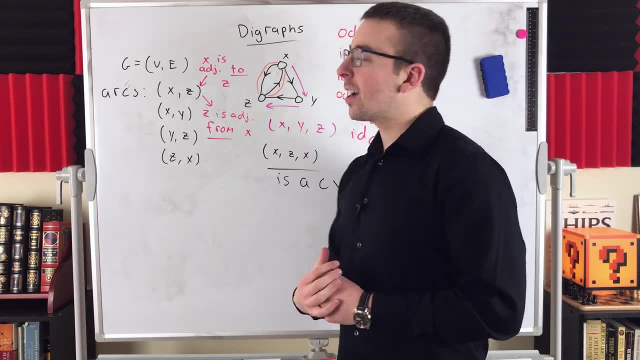 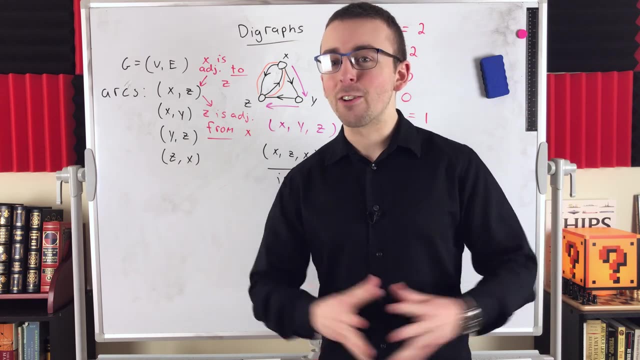 vertices in a graph, We will get two times the number of edges in the graph. What do you think the analogous result is for directed graphs Turns out. in a way it's even simpler than the original first theorem of graph theory. We call it the first theorem of digraph theory. So let me know. 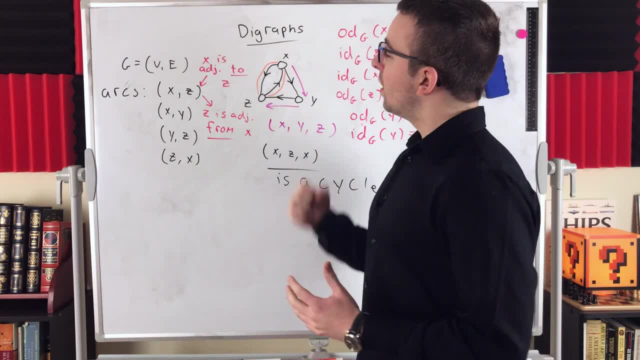 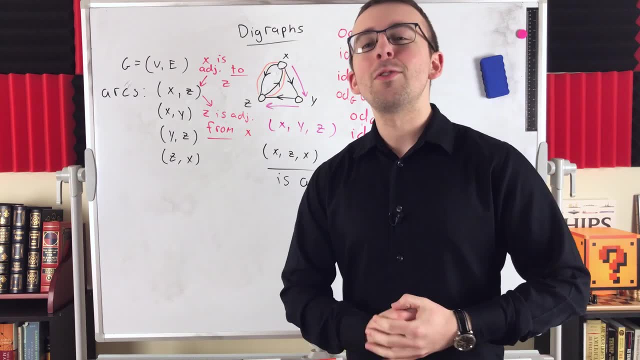 what you think about those two things down in the comments And I hope this video helped you understand a bit about digraphs and how we describe them. Running out of breath: Let me know in the comments if you have any questions. If you have any questions, let me know in the 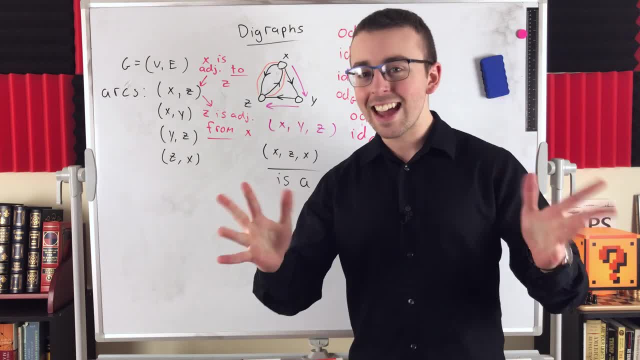 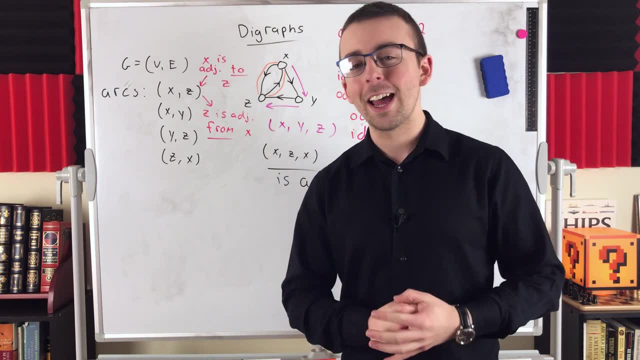 questions, Need anything clarified or have any other video requests? Thank you very much for watching. I will see you next time and be sure to subscribe to the Swankiest Math Lessons on the internet. And a big thanks to Valo who, upon my request, kindly gave me permission to use his 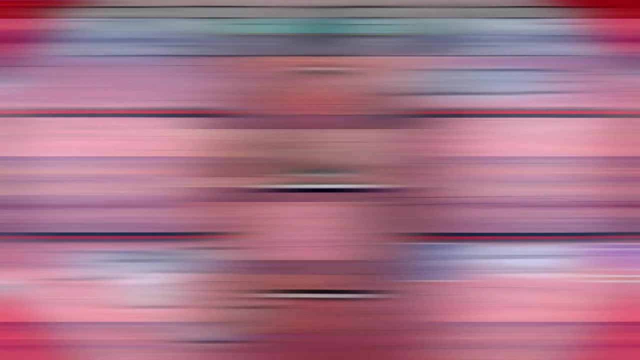 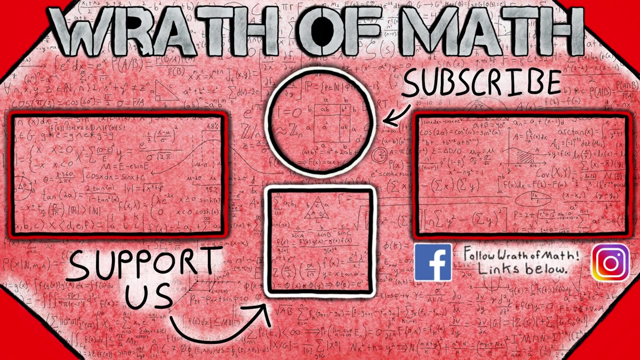 music in my math lessons Link to his music in the description. Thank you very much for watching this video. I hope you enjoyed it. See you next time.